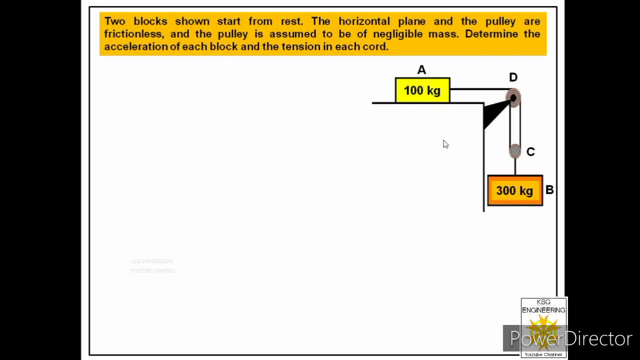 And we are asked to find acceleration of each block, That is, of block A and block B. That means we have to find AA and AB And we have to find tension in each chord. So we have to find tension in these four chords. 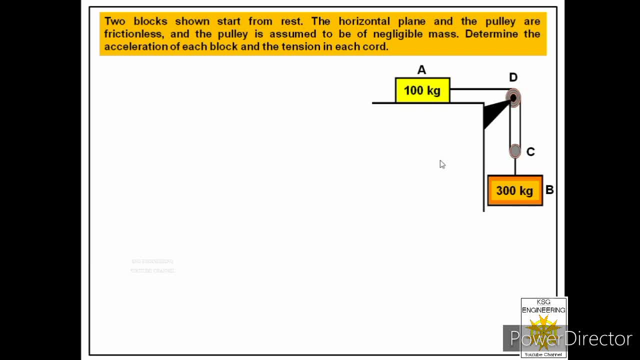 Shown to us And it is mentioned that the horizontal plane and the pulley are frictionless Means there is no friction And the pulley is assumed to be of negligible mass. It means we have to consider mass of the pulley equal to zero. 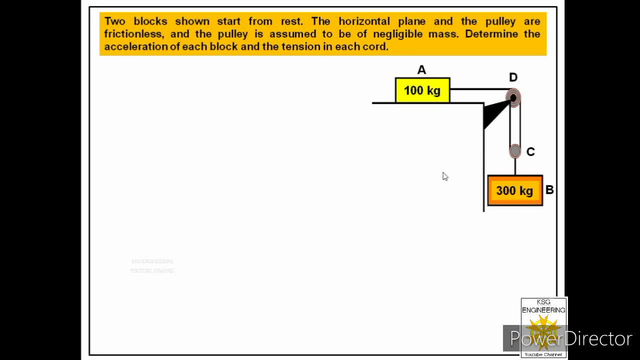 So in order to solve this problem, we have to first see how many free bodies we have to draw. So if you will see carefully, You will find that in this problem there are three bodies which are in motion: Block A, block B and pulley C. 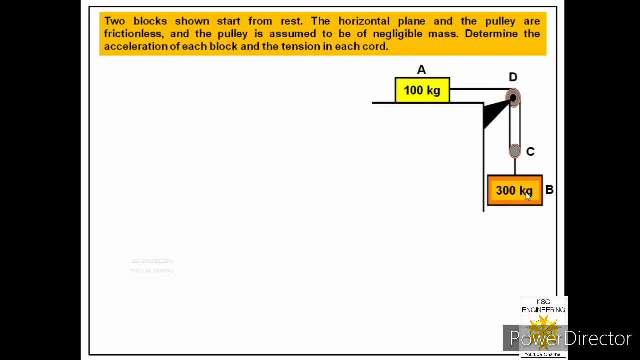 It means we have to draw free body of these three in this particular problem. So let us first start with block A. So let us construct its free body. After that we will observe its motion. So let us construct free body of block A. 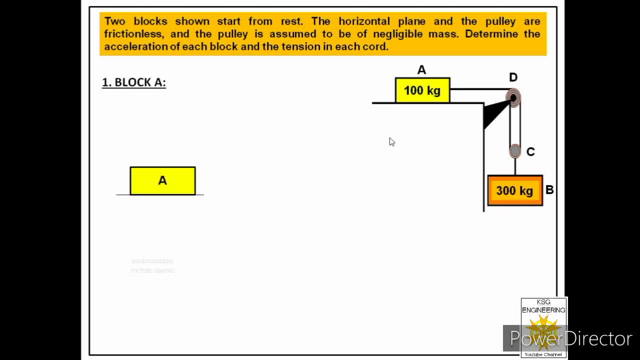 So, in order to construct the free body of block A, first of all we will represent that block on the horizontal surface And after that we will label the forces. So the first force which we should label is the weight of the block, And we are given mass of the block as 100 kg. 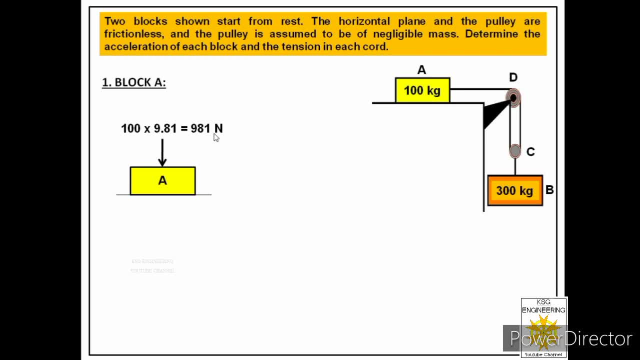 So we will multiply that with 9.81 to get its weight, which will be 981 N, And weight will always act in downward direction. After this we will show the normal pressure which will act normal to the horizontal surface on which this block is resting. 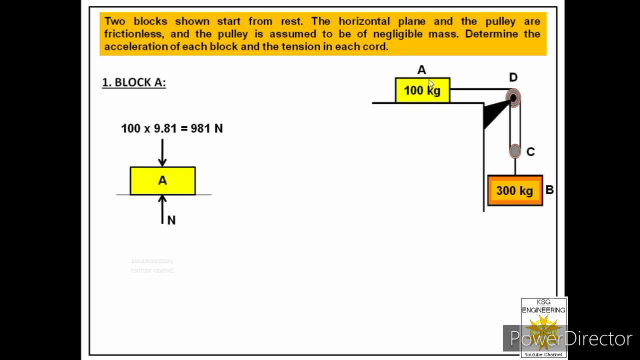 Then in this particular diagram we are shown that this block is connected to a cable And this is a block of 300 kg. It will move in downward direction, So block A will move towards right, So there will be tension in this cable towards right. 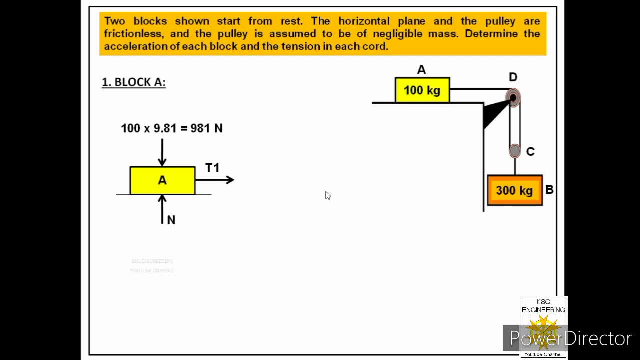 So let us show that tension now. So in the free body of block A we have to show that tension towards right. So let us call that as T1.. Now over here in this question it is written that the surface, horizontal surface and the pulley are frictionless. 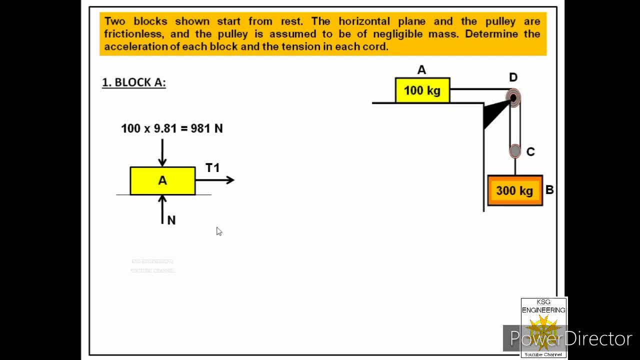 It means there is no friction force acting in this free body. It means these are the only forces which are acting on block A And we are ready with the free body of block A. Now let us see the motion of block A. Now in this question we are asked to find acceleration of each block. 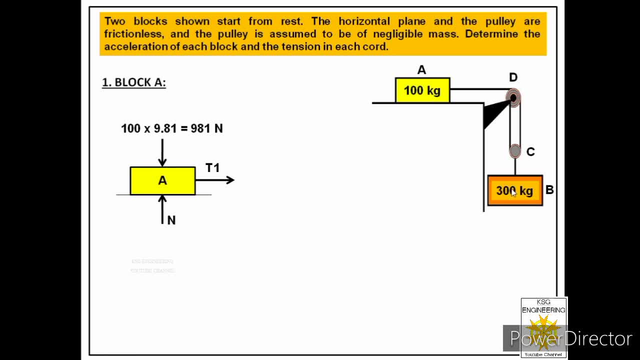 It means both the blocks are moving And this block is of 300 kg. It will move down, which will make this block to move towards right. So it means whatever forces are acting on block A, these forces are responsible for the acceleration of block A. 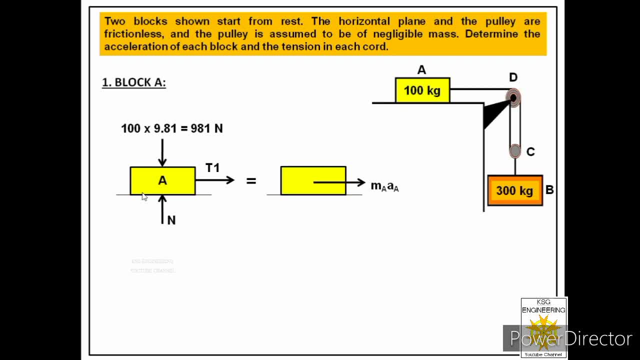 So we can say: summation f is equal to ma. So over here ma is representing mass of block A, aa is the acceleration of block A. So we have concluded that block A is moving towards right with an acceleration of aa. So it means we can use first equation, that is from Newton's second law. 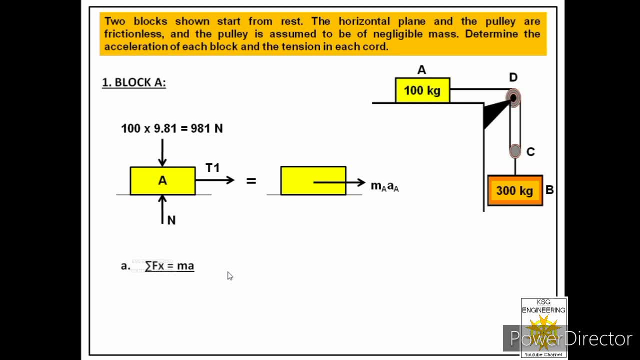 Summation: fx is equal to ma, So let us see how many forces are acting in x direction. So there is only one force labelled as T1 over here which is acting in x direction. So this equation will reduce to: T1 is equal to ma aa. 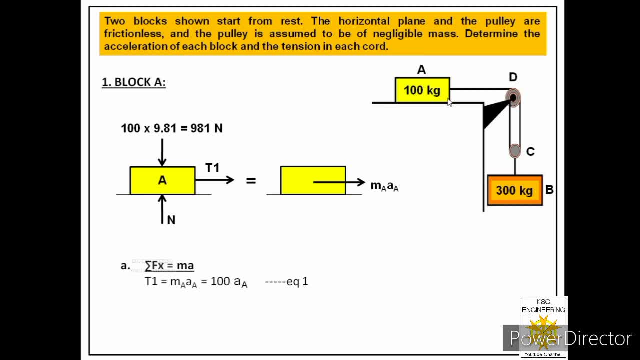 And we are given mass of block A as 100 kg. So we will replace ma by 100.. So equation will be equal to: T1 is equal to 100 kg. Now in this equation we have two unknowns: T1 and aa. 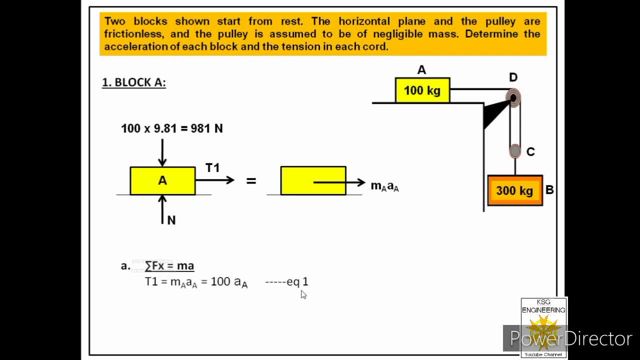 So we cannot solve it. So let us call this equation as equation number 1 for time being. Let us move to the second block. Now we will draw the free body of second block, that is, block B, And we will understand its motion. 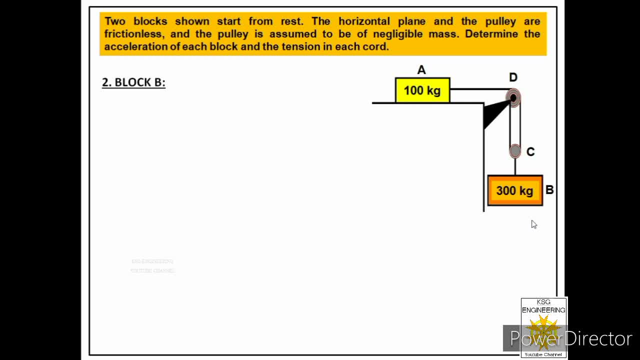 So let us draw the free body of block B. So in order to draw the free body of block B, we have to first represent the block, And first force which we will show in this free body is the weight of the block. We are given mass of the block as 300 kg. 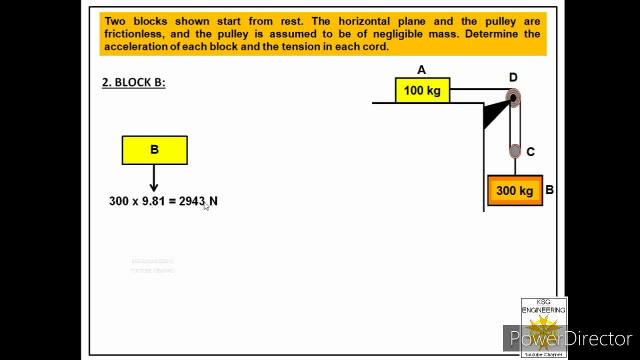 So we will multiply it by 9.81 to get its weight. That will be 2943 N And we have to show it in downward direction in the free body. And we know this block is connected with the help of a cable over here. 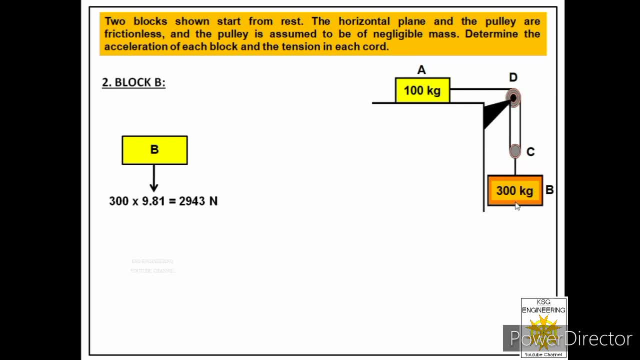 So in the free body of block B we will show weight in downward direction And that weight will be balanced by tension in this cable. So let us represent that tension as T2.. So in the free body of block B there are only two forces acting. 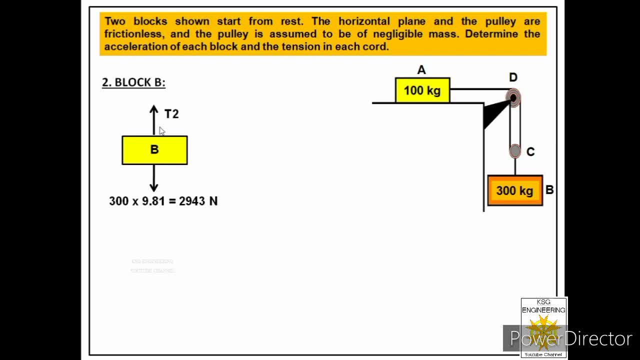 One is the weight of block B acting in downward direction. Second is tension in the cable connected to block B, which will act in upward direction. Now we know this block is moving in downward direction, So it means this system of forces is responsible for the acceleration of the block in downward direction. 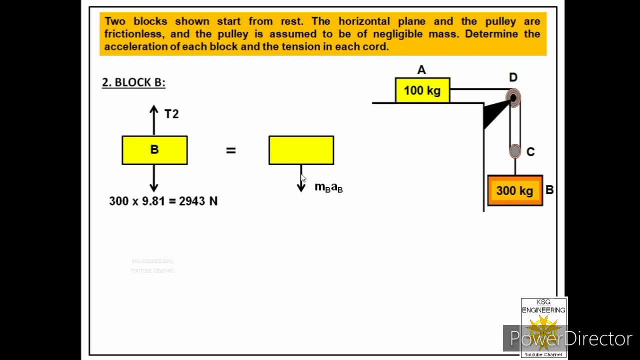 So we will say: summation F is equal to mBab. So over here we will apply the first equation, that is Newton's second law. Summation Fy is equal to mA. Now let us see how many forces are acting in y direction. 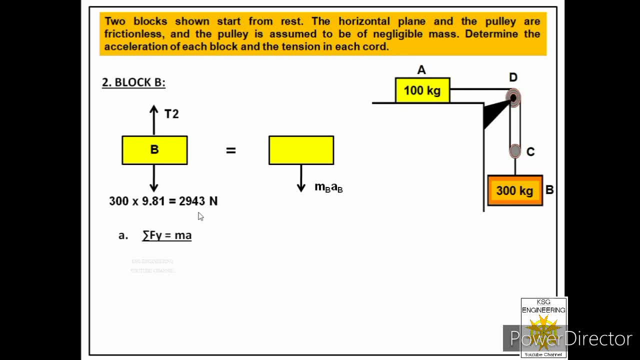 So there are two forces. One is weight of the block, Second is tension in the cable. Now we will consider that force positive, which will act in the direction of motion. Now, weight is acting in the direction of motion, So we will consider this as positive. 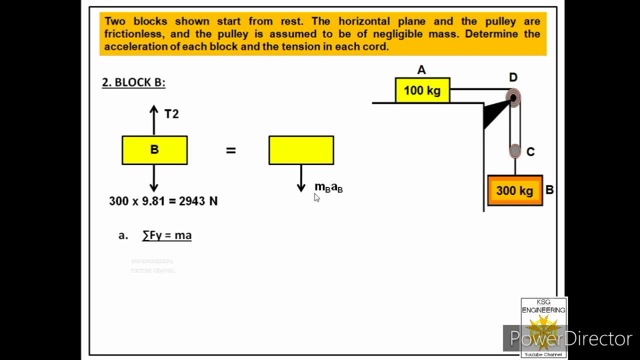 And tension is acting opposite to the direction of motion. We will consider that as negative. It means our equation will be minus T2. plus 2943 is equal to mBab, So this equation will further reduce to T2 equal to minus 300ab. 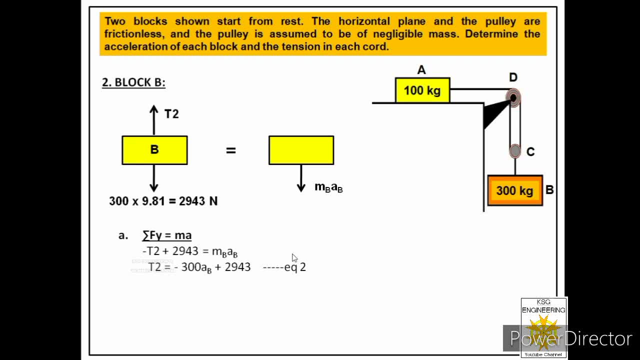 where 300 represents the mass of block B plus 2943.. So in this equation we have two unknowns. One is tension in the cable T2.. Second is acceleration of the block AB. So we cannot solve this equation. So let us call this equation as equation number 2 for time being. 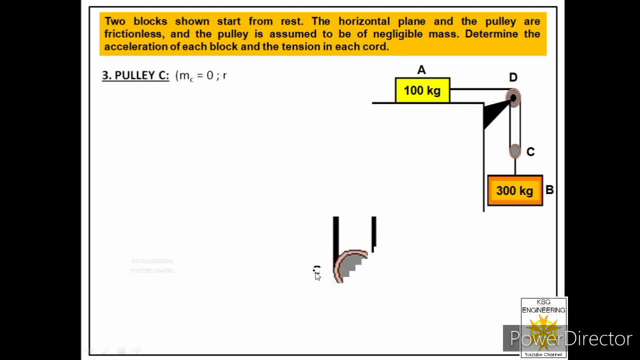 Now we will consider the third body in this problem, that is, the pulley. Now it is mentioned in the problem that pulley has a negligible mass, So it means we will consider mC is equal to 0. Now let us draw the free body of this pulley. 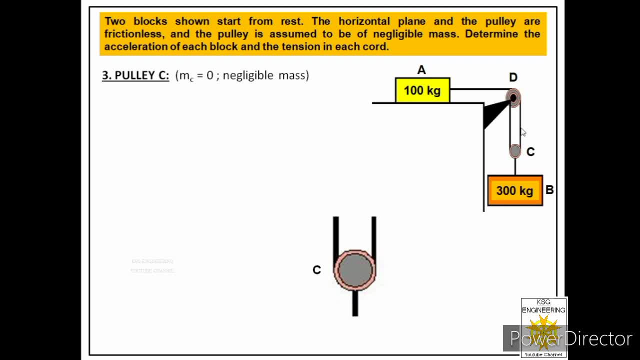 And let us observe its motion. So, in order to draw its free body, we have to consider pulley And we have to consider three cables Attached to that pulley. One is connected to block B And second is wrapped around the pulley. 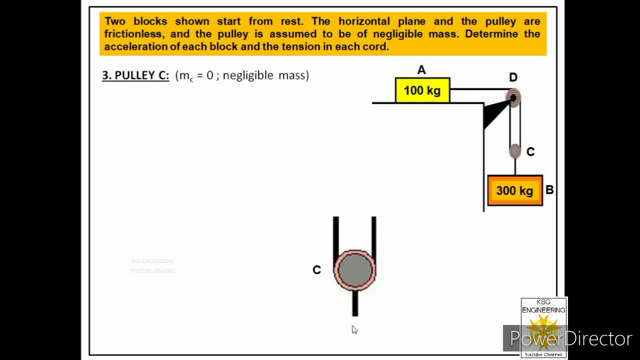 So we have shown these cables over here. Now let us show the tensions in these cables. In this cable we know tension will act in downward direction Because this cable is attached to block B, Which has a mass of 300 kg. So it will pull that cable in downward direction. 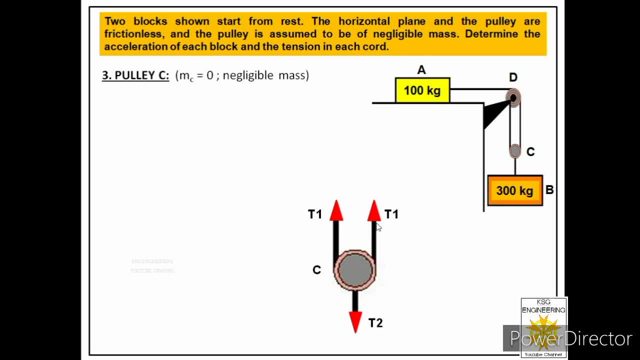 And in these two cords tension will act in upward direction, Which will balance this pulley. And these tensions will be T1 only Because this cable is connected to block A, So same tension will be there throughout in this cable. Now let us see its motion. 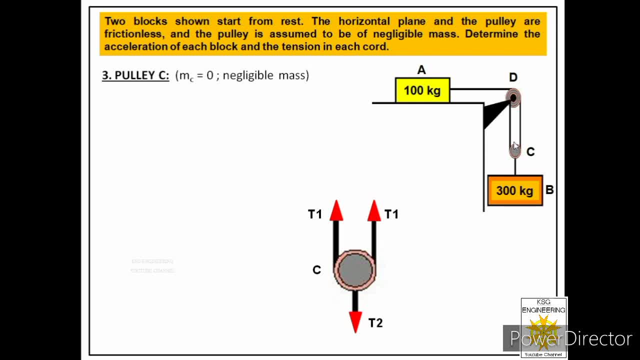 Now, when block B will move in downward direction, This pulley will also move in downward direction. But over here it is mentioned that we have to assume mass of pulley as 0. So it means this summation Fy will reduce to 0.. 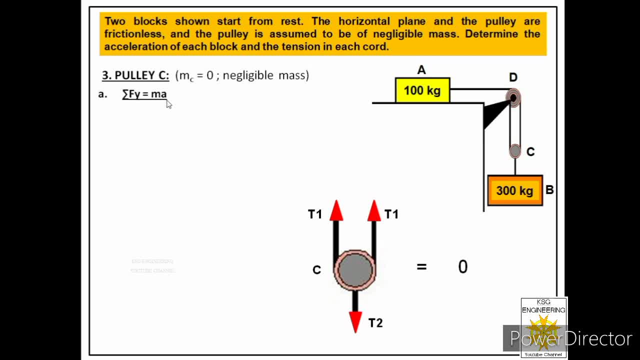 So we will apply equation Summation Fy is equal to Ma. But over here in this question we are given that we have to consider mass of the pulley, 0. So this equation will reduce to summation Fy equal to 0.. 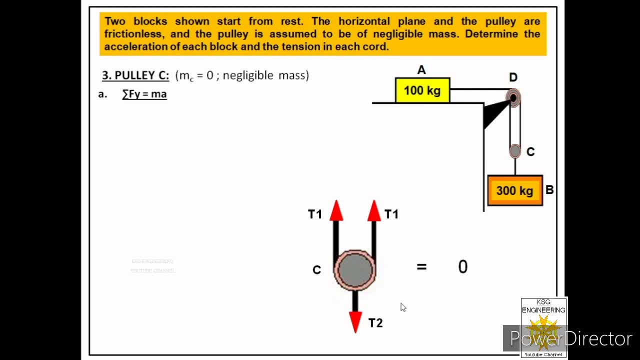 Now let us see how many forces are acting in y direction. So there are three forces. One is T2, acting in downward direction, Which is acting in the direction of motion, So we will consider this as positive. Other two tensions are acting in upward direction. 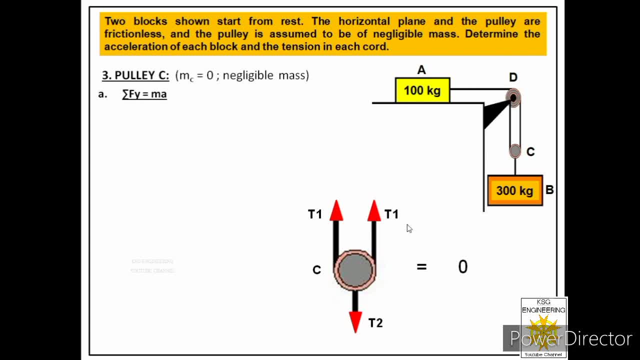 Which is opposite to the direction of motion. So we will consider these two negative. It means final equation will be: T2 minus 2T1 is equal to McAc, But Mc is given to us as 0. So this equation will reduce to T2 minus 2T1. 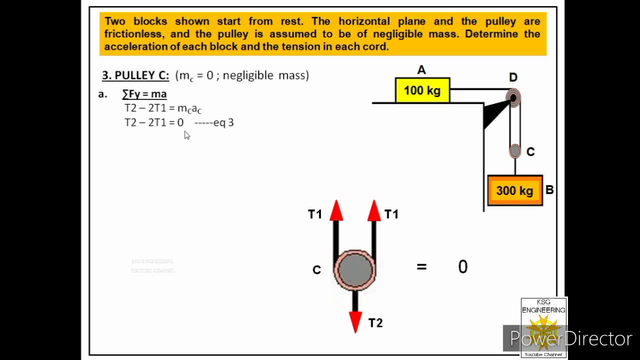 Which is opposite to T1 minus 2T1 is equal to 0.. Now in this equation we have tension T2 and tension T1. And we have already found the values of T2 and T1 in the free body of block A and in the free body of block B. 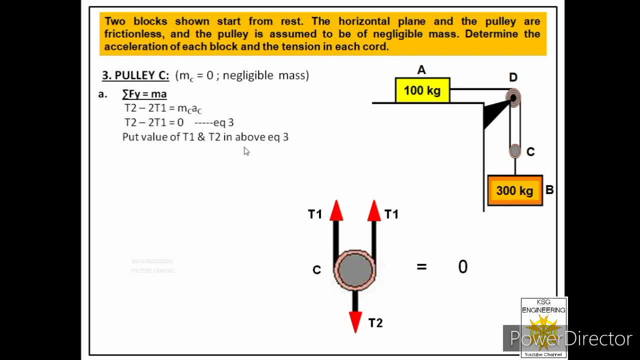 So we will say: put value of T1 and T2 calculated in the free body of block A and block B in above equation, Then we will get equation as Minus 300ab, plus 2943, minus 2 into 100aa equal to 0.. 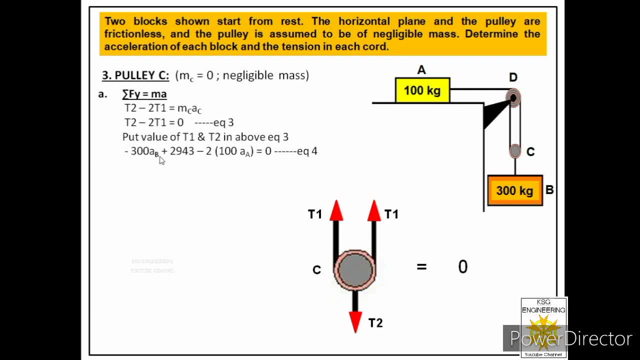 Over here. in this equation we have still two unknowns, So it means we cannot solve this equation. So we have to find a relation between these two accelerations In order to get only one unknown in this equation. So let us see what relation we can find between these two accelerations. 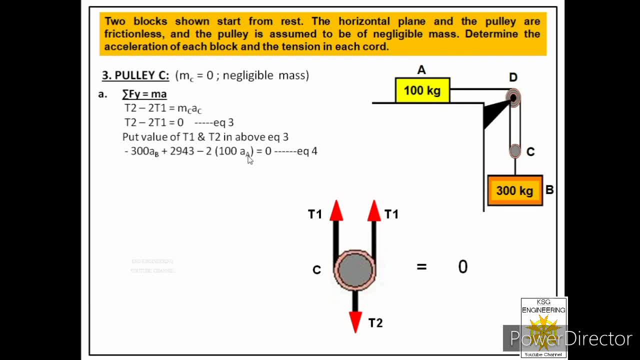 Means between acceleration of block B and acceleration of block A. So for that we have to understand the motion again. Now let us see what is happening over here. When block B will move in downward direction, Then block A will move towards right. And let us suppose block A has moved by x units towards right. 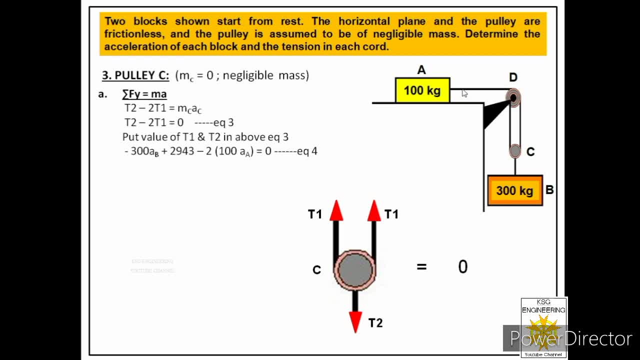 That means if this cable Has moved by x units towards right, Then that length of the cable is wrapped around this pulley And because of this block B will move only half of the distance moved by block A. So we can say the distance travelled by block B is half the distance travelled by block A. 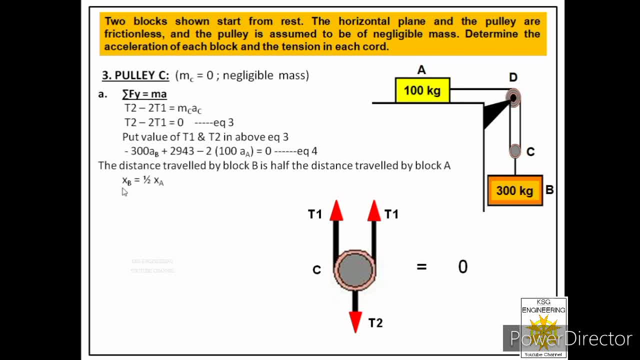 So we can say: if xB is the distance travelled by block B And xA is the distance travelled by block A, Then xB will be equal to half xA, And when we will take double derivative of this equation, We will get acceleration of block B equal to half the acceleration of block A.